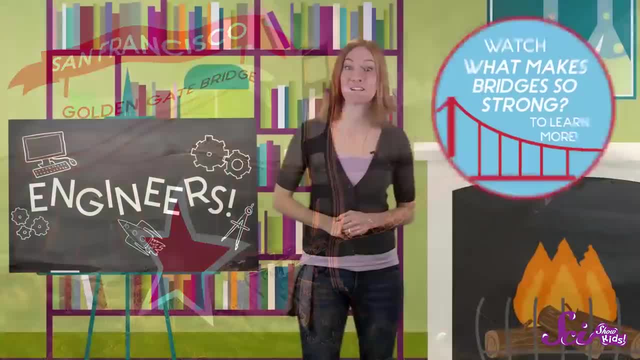 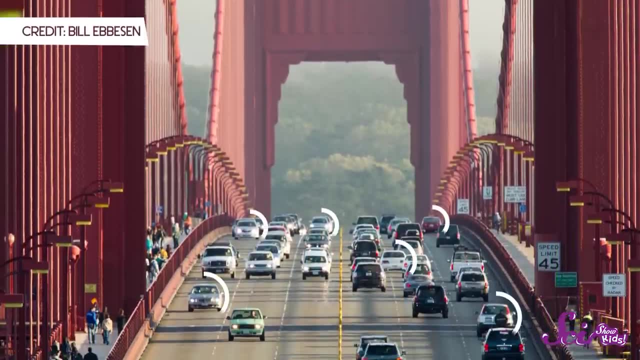 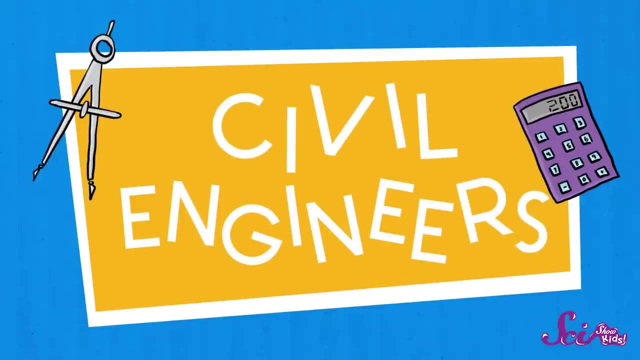 other towns on the mainland And we've studied that bridge here on SciShow Kids because it's a great example of how bridges can be so big and still be strong enough to carry thousands of cars, trucks and people. Now the Golden Gate Bridge was the work of a special kind of engineers called civil. 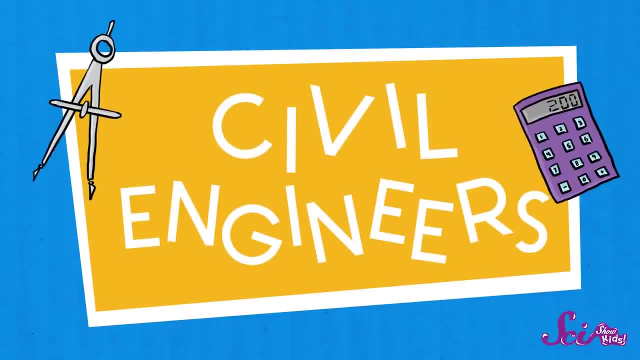 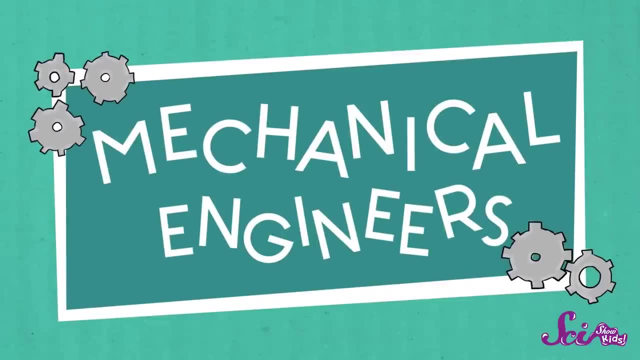 engineers. They designed big things that are used by lots of people, like buildings, roads and bridges. But there are lots of other kinds of engineers too. Mechanical engineers make things like tools, engines and machines- Machines like bikes and cars. 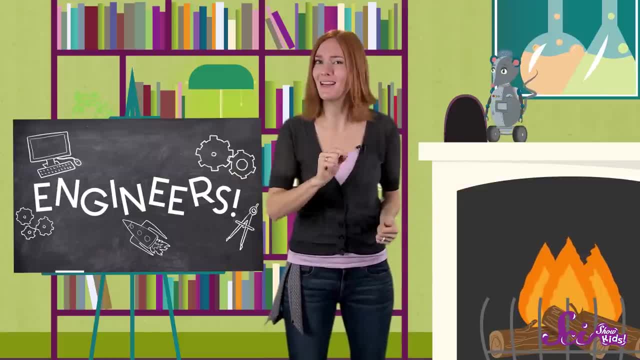 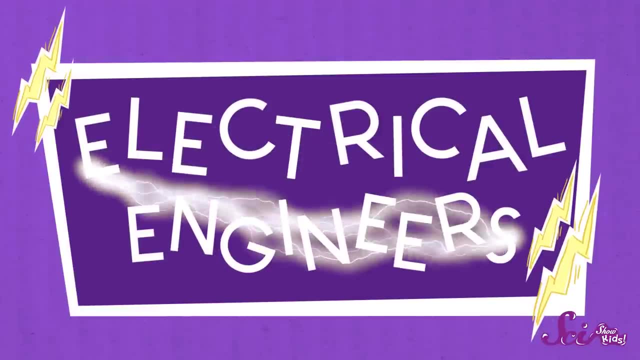 If your problem is not being able to get from one place to another quickly, bikes and cars are solutions to that problem. Then there are electrical engineers. They study electricity and design things that use it, like, say, the microwave in your kitchen. If your problem is cold food, then microwaves. 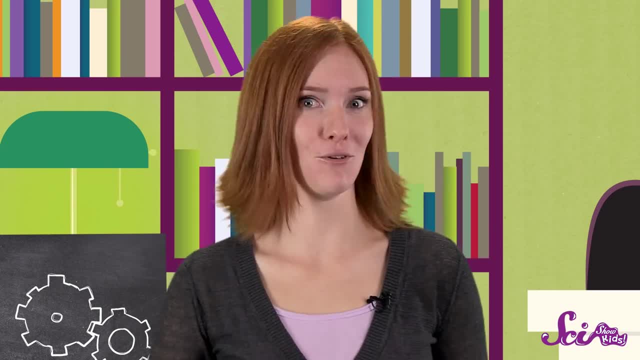 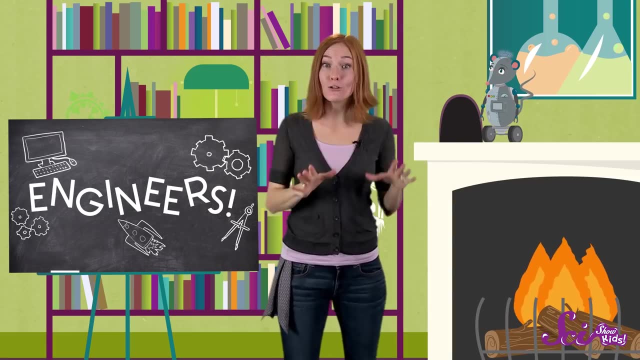 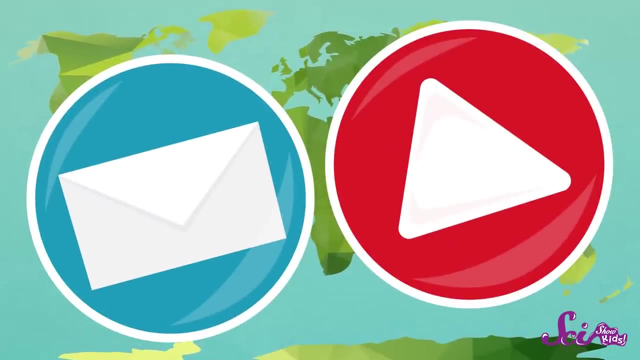 can solve that problem too, But don't forget about computers. Software engineers are people who work on computers to make them faster and able to do more things, And computers solve all kinds of problems like connecting people in faraway places by email and video and providing information on certain topics like engineering to people. 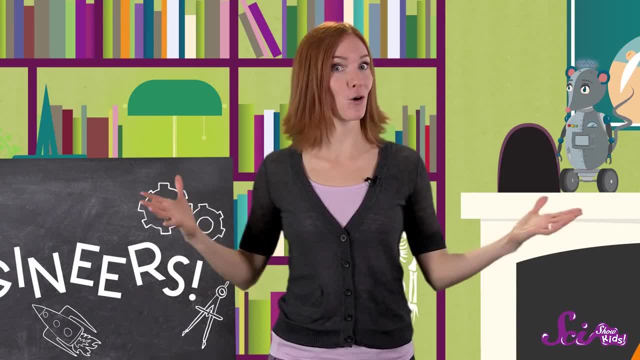 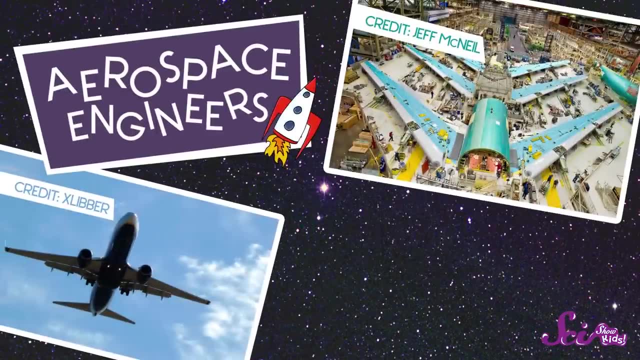 like you who want to learn more about them, And if you're interested in exploring space, then you're definitely going to want to know all about aerospace engineers. They're the people who design and build airplanes and spaceships. If your problem is that you're stuck on Earth, well, they can help you with that. 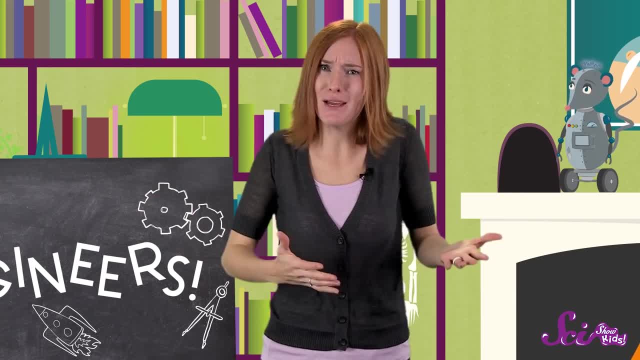 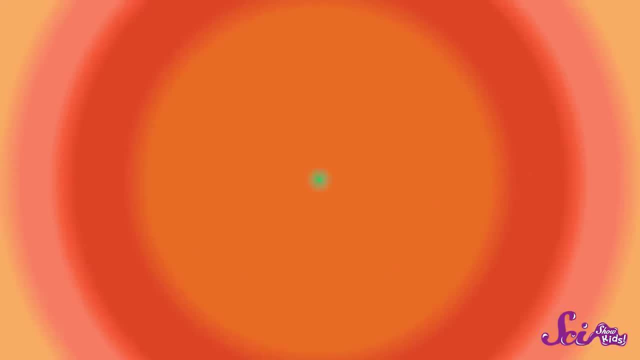 Over a hundred years ago we didn't have aerospace engineers because we didn't have any airplanes or spaceships. But today we do, thanks to the people who engineered them. Who knows what things will need engineered in another hundred years? What kind of engineers? 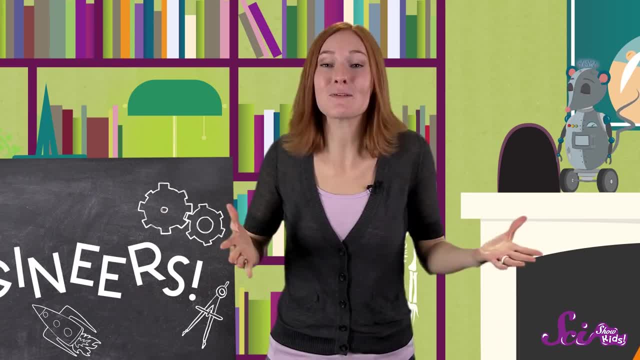 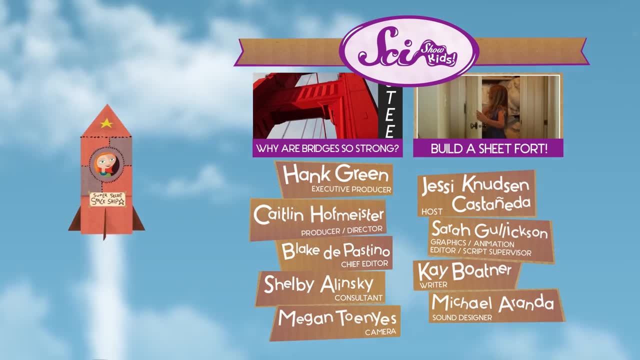 do you imagine in the future? Let us know by getting a grown-up to help you. leave a comment or email us at kids at the SciShow dot com. Thanks for learning about engineers with us and we'll see you next time. Thanks for watching and we'll see you next time.